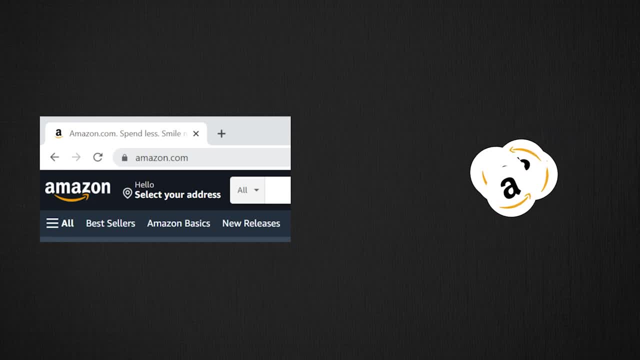 server. It has many servers but for the sake of simplicity we will refer Amazon as a single server here. Now, your client doesn't necessarily need to know what Amazon server is. It just knows that it's a server it can talk to or send requests to. It will request information to the server. 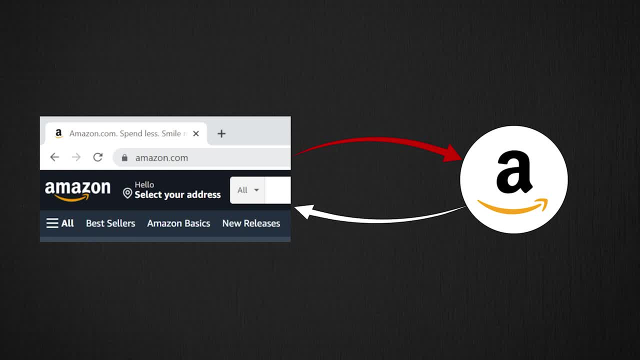 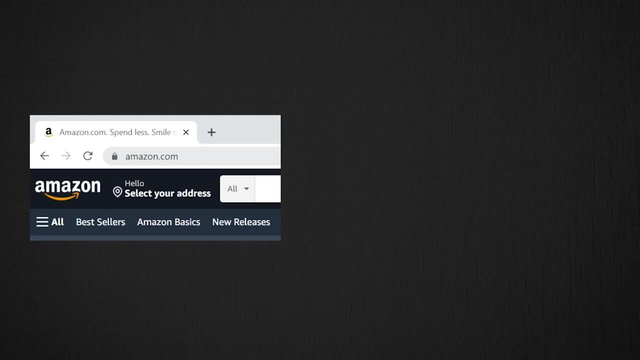 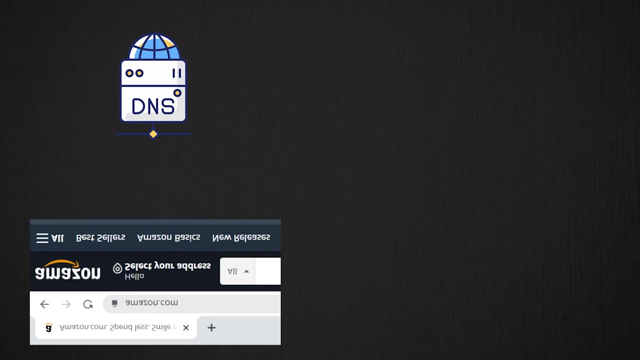 and, based on the response from the server, it will be able to do other stuff. So when you type amazoncom in the browser, your browser doesn't even know how to talk to amazoncom or the server Behind the scenes. it makes a DNS query to find the IP address of amazoncom server. 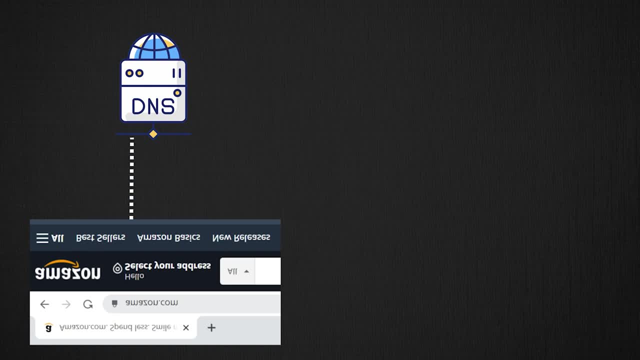 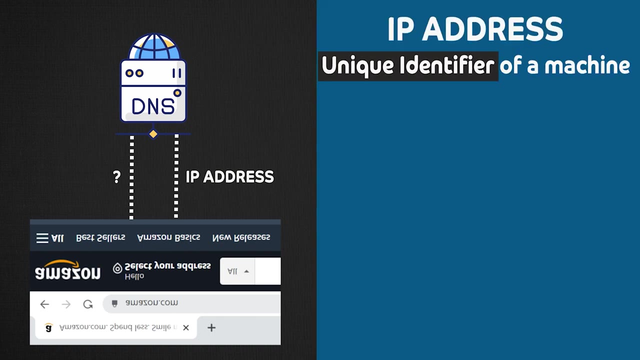 You may think of DNS query like a special request that goes to a predetermined set of DNS servers which basically says: hey, what is the IP address of amazoncom? The DNS servers returns back the IP address. Think of IP address as a unique identifier of a machine: All computers which 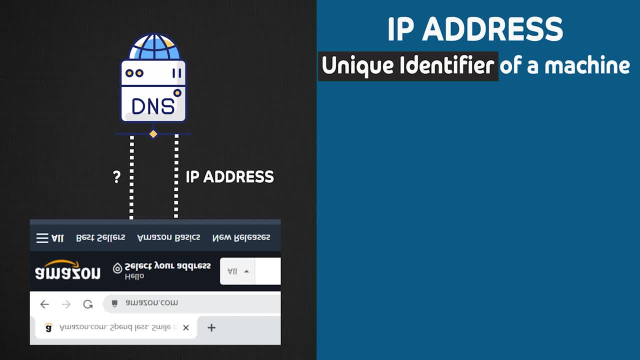 are connected to the internet can discover these public IP addresses and send data of packets of information in terms of bytes, to these IP addresses. IP addresses can be thought of as a mailbox granted by certain authority, So in case of amazoncom, amazon web services, 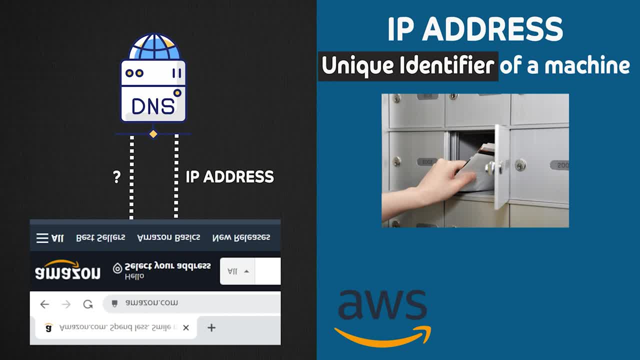 the cloud provider is the entity that has granted IP address to amazoncom. Now if you build your own server, let's say in Google cloud, Google cloud provider will be the entity that will grant your server IP address. For example, in windows computer, if you open command prompt and type 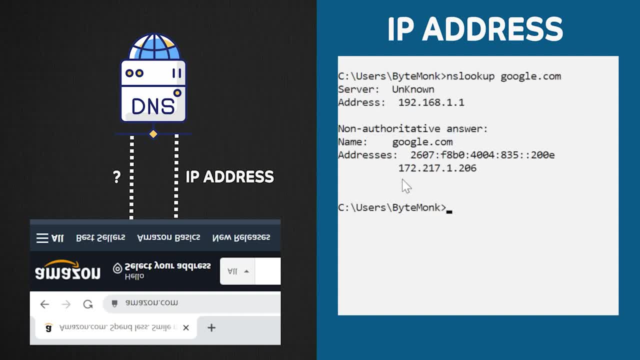 nslookup, you will get the IP address of amazoncom. Now if you build your own server, let's say in google cloud, googlecom, it will return the IP address of google servers. If you run the same nslookup command again, you will get a different IP address, because google has got many servers. 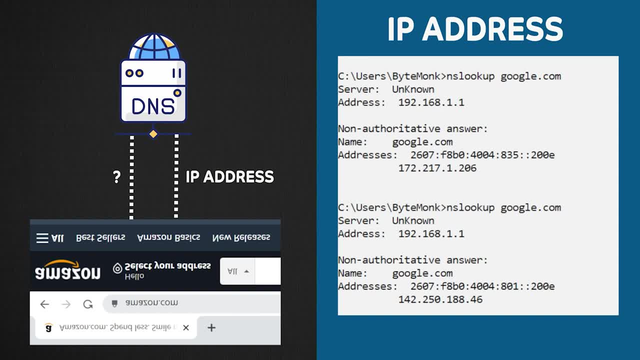 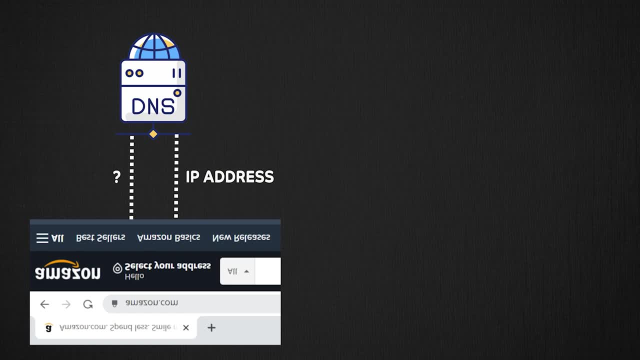 and whichever server is available, IP address of that server will be returned. If you are in a mac, you can use the command dig. So now your browser made the DNS query. It now knows the IP address of the server and is now ready to send requests to your servers. It then sends an HTTP request. 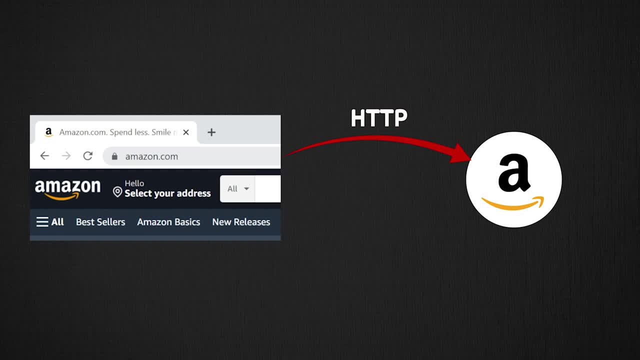 to the server. Now I have covered HTTP in another video, But for now just think of HTTP a way to send information which a server can understand. So when we say your browser or client send a request to the server, it means that it sends a bytes, or 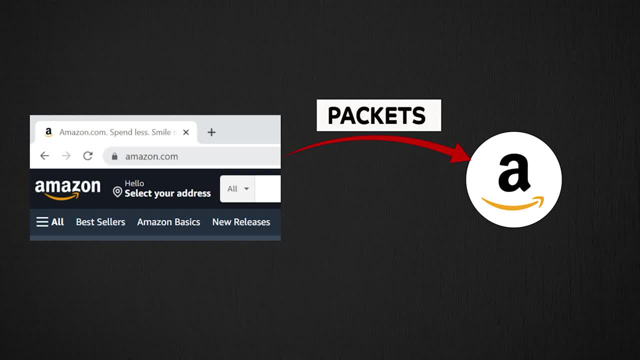 characters packed into what we call packets in some special format. This request will also contain IP address of your browser or your machine, also called the source IP address of the request. So when the server gets the request, it knows which IP address it needs to send response to. 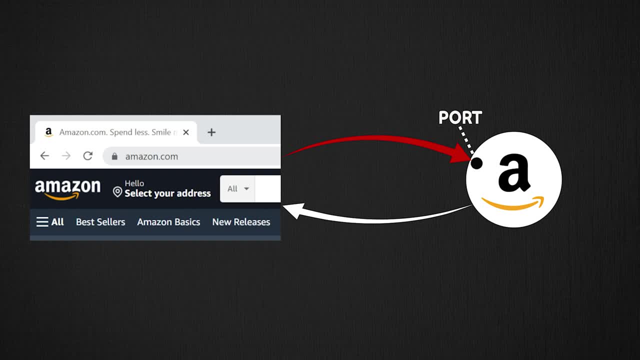 A server listens to a request and it knows which IP address it needs to send response to. This is for client requests on specific ports. In fact, any machine which has an IP address has got 16,000 ports that programs on the machine can listen to. So, as a client, when you're. 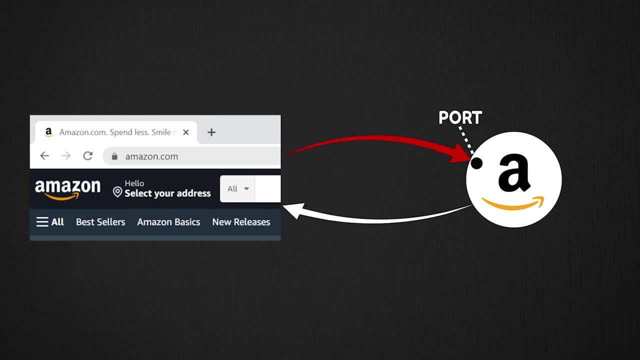 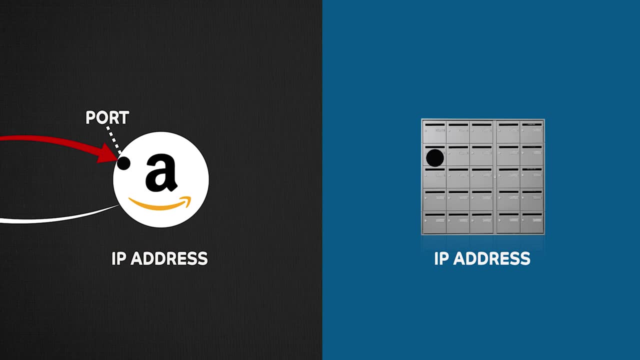 communicating with a server, you need to specify the server port you want to communicate on. You can think of IP address as a mailbox to an apartment complex and think of ports as the actual apartment number. Typically in a client server model, client usually knows the port they. 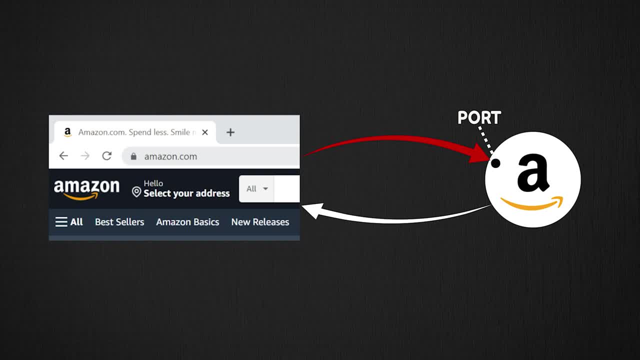 need to use, depending on the protocol they are trying to speak to the server. For example, if a client is going to speak to a server using HTTP protocol, it will always going to use port 80.. For HTTPS, it is port 8443.. Check out my video on network protocols to understand further. 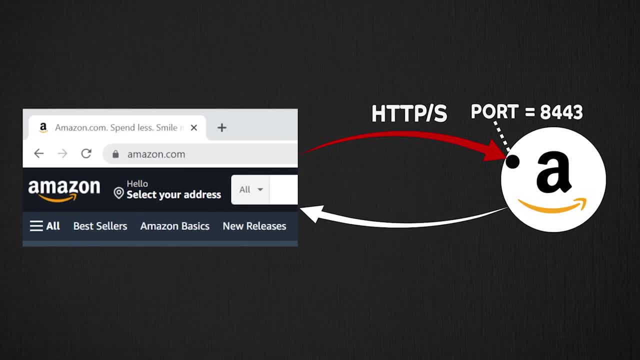 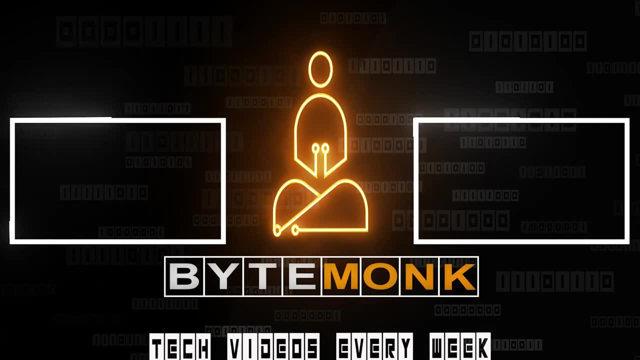 And if you have found this video informative, please give a thumbs up and consider subscribing. Thank you. 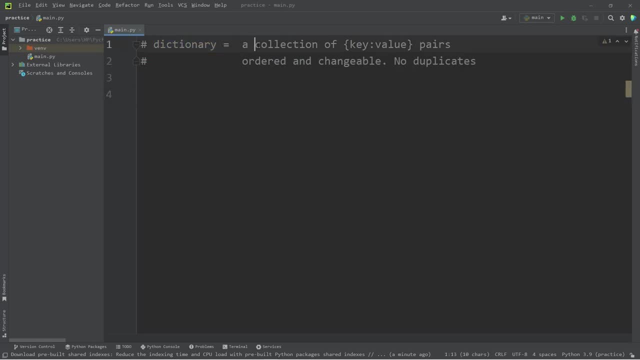 Hey everybody, in today's video I'm going to explain dictionaries. A dictionary is one of the four basic collection types for beginners. A dictionary consists of key-value pairs. They are ordered and changeable. No duplicates allowed. A few examples of key-value pairs could be an ID and a name, an item and a price. 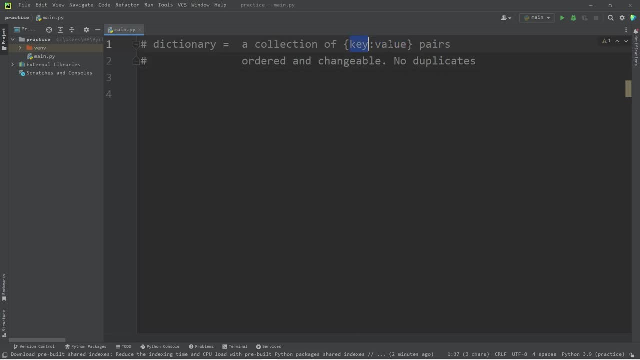 But in today's example we'll create a dictionary of countries and capitals. Let's name our dictionary Capitals. Capitals equals: Enclose your dictionary with a set of curly braces, much like what you do with sets. The first country will be the USA To add a value to this key type colon.